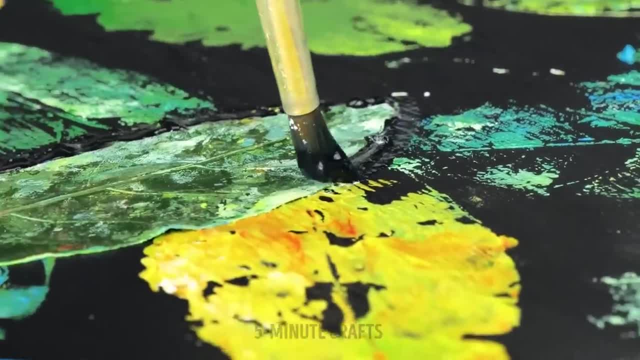 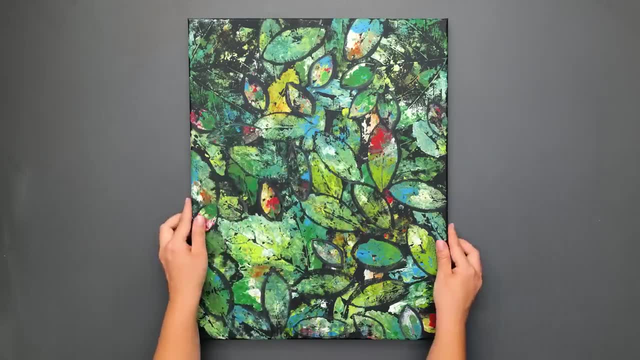 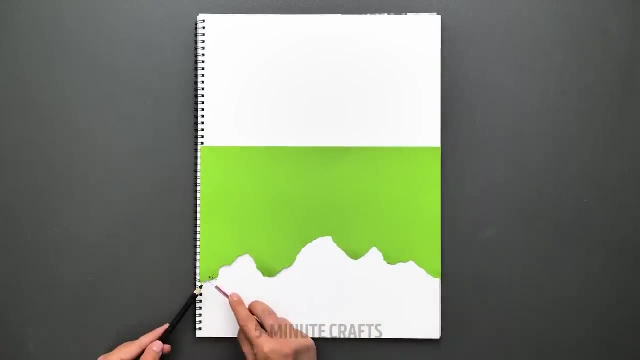 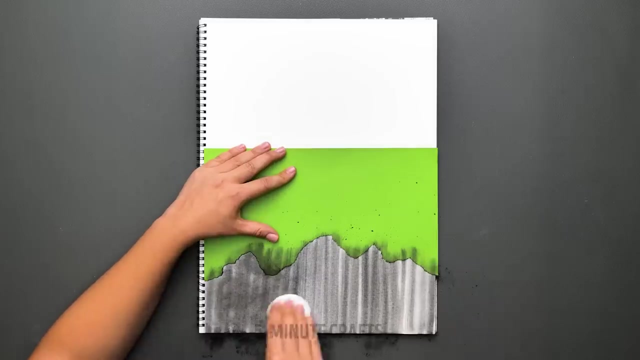 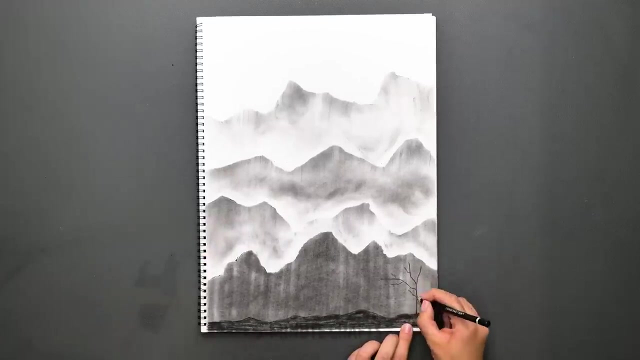 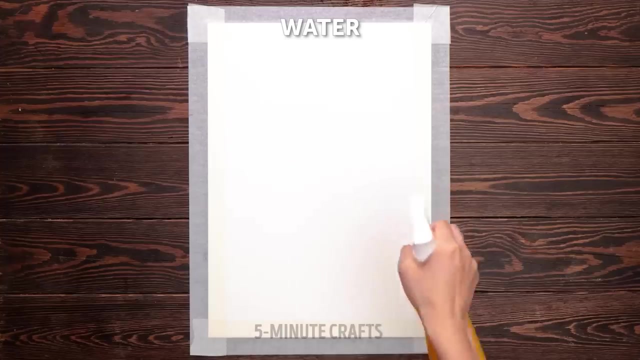 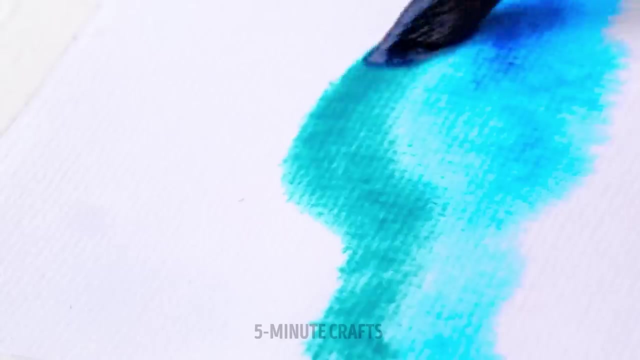 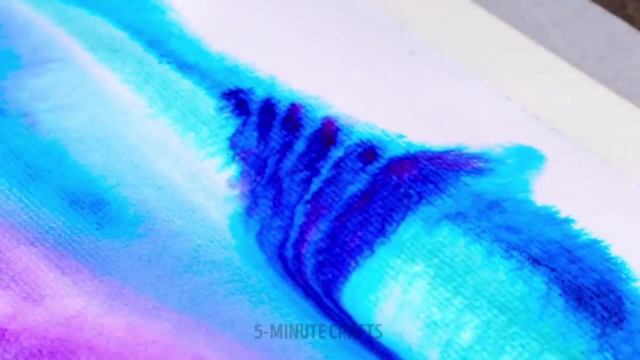 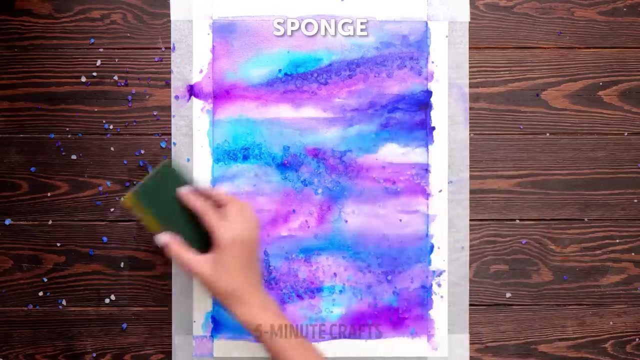 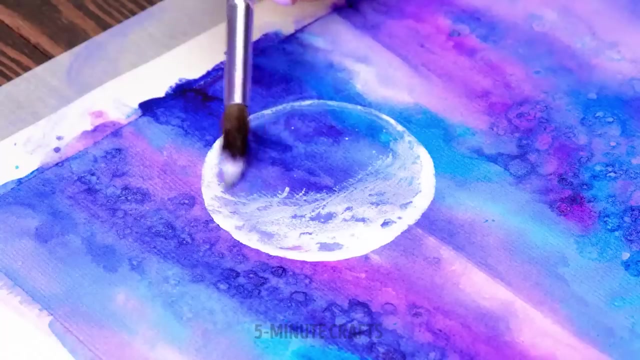 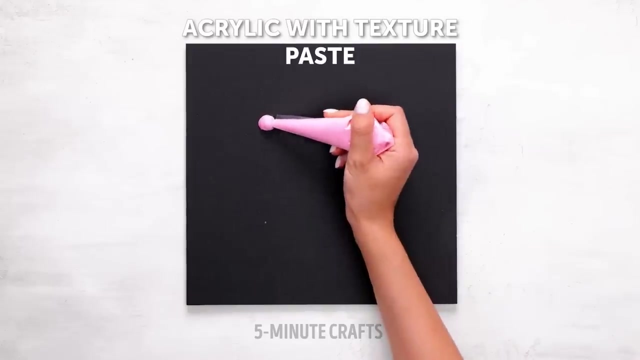 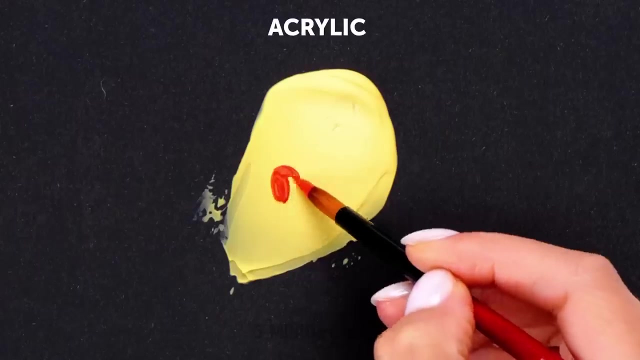 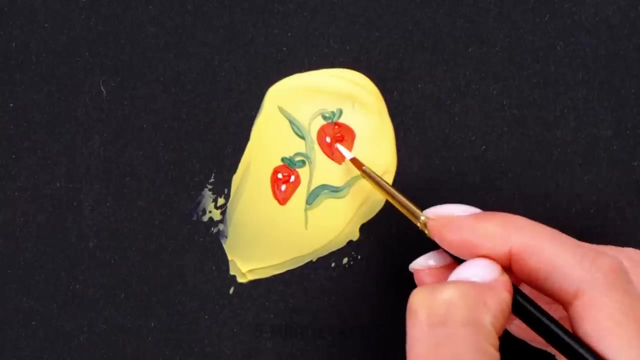 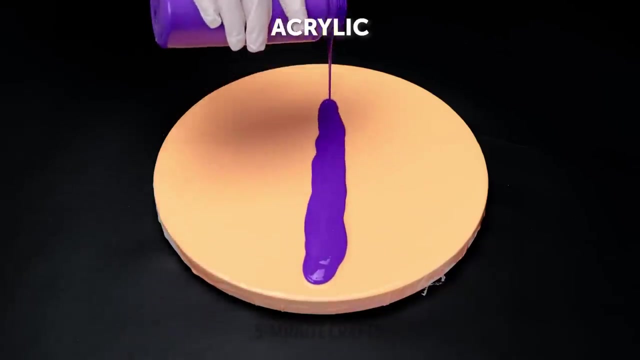 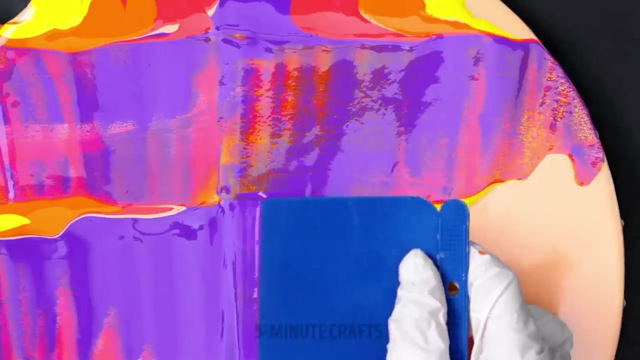 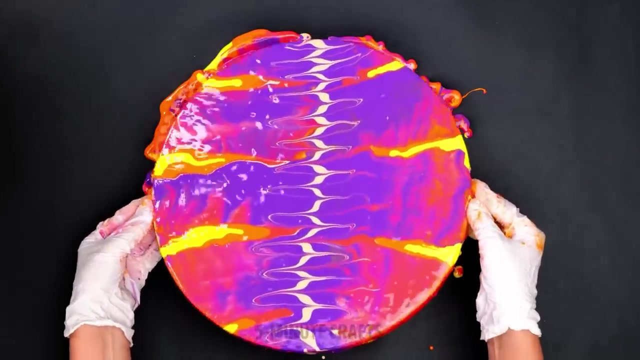 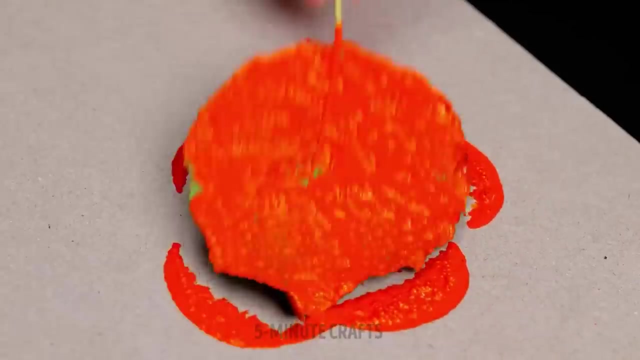 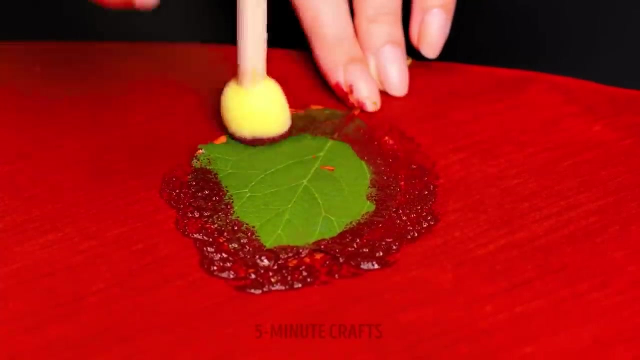 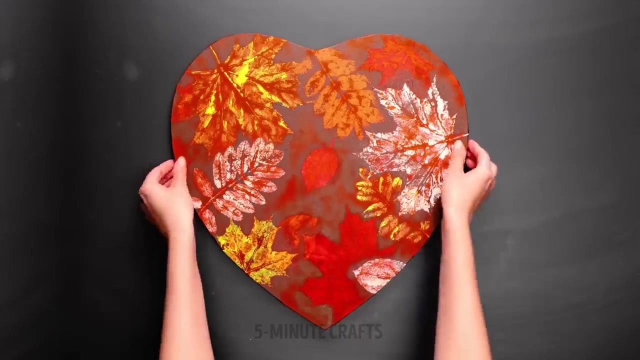 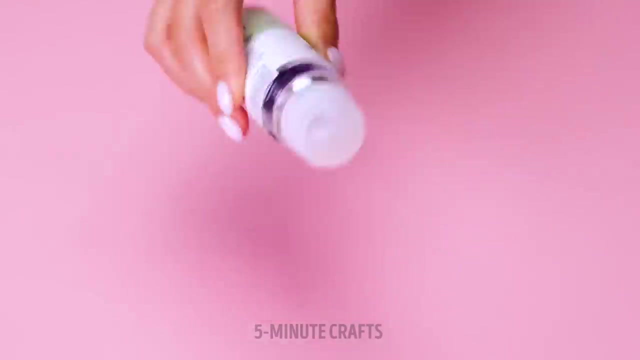 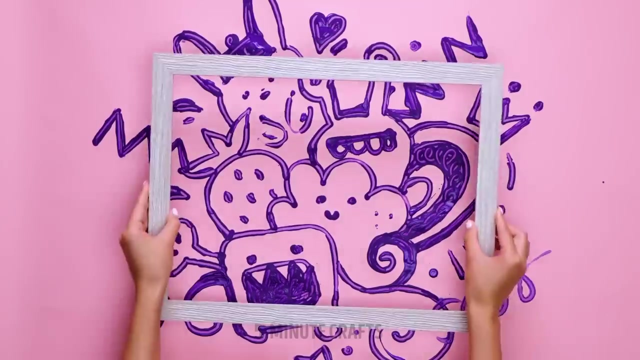 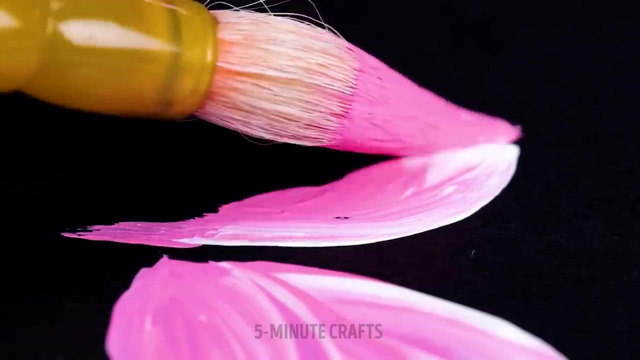 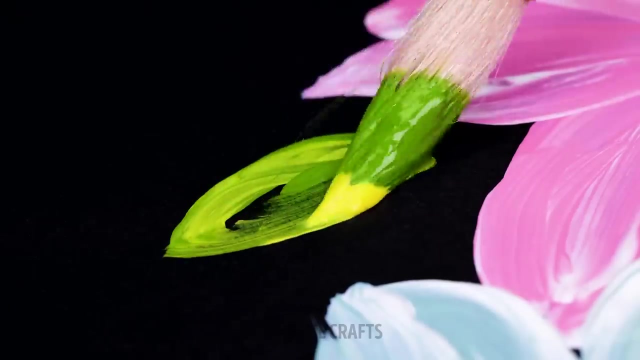 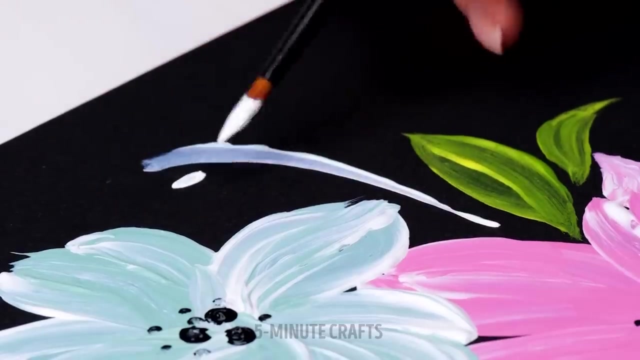 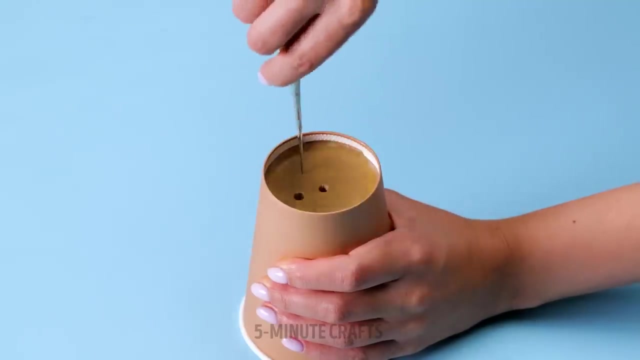 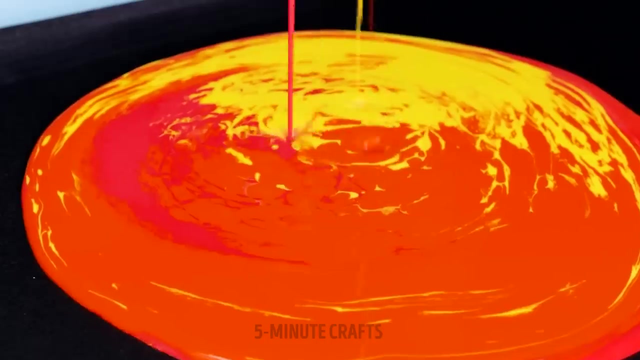 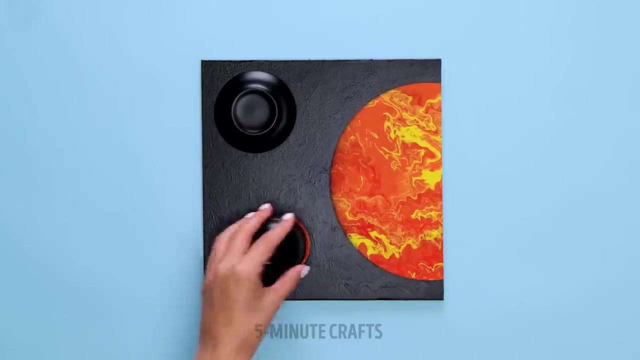 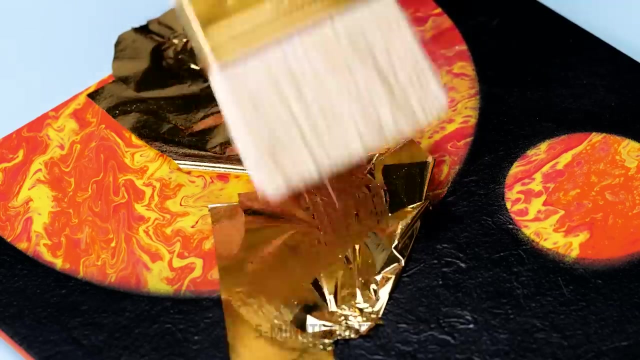 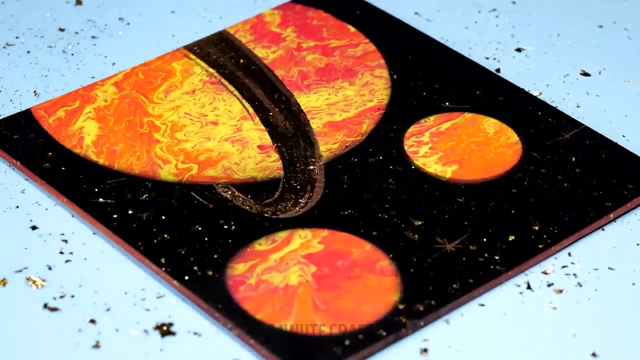 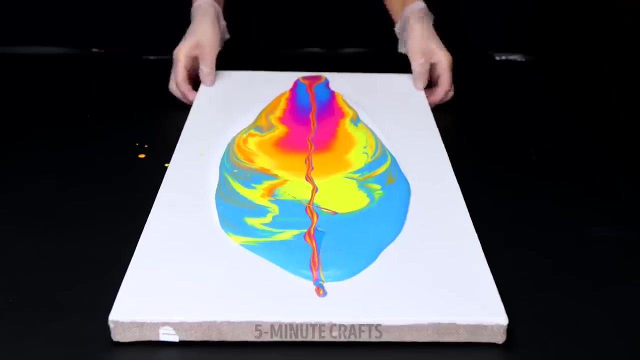 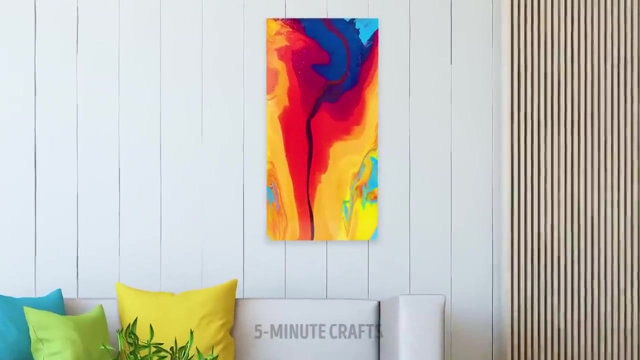 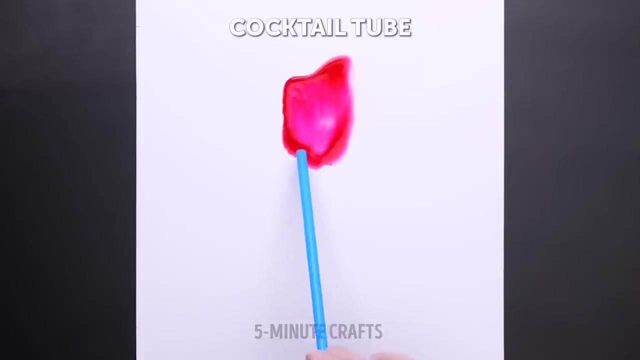 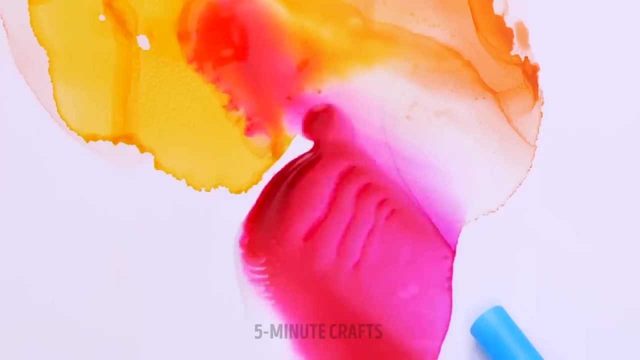 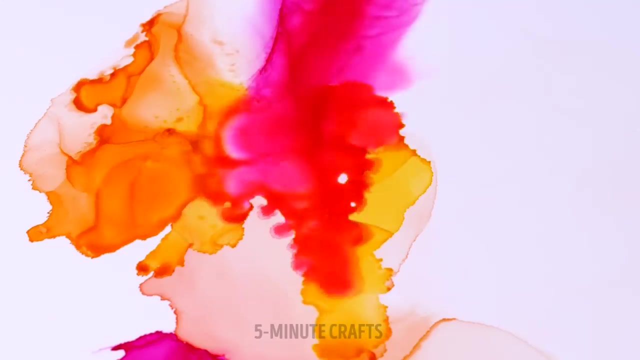 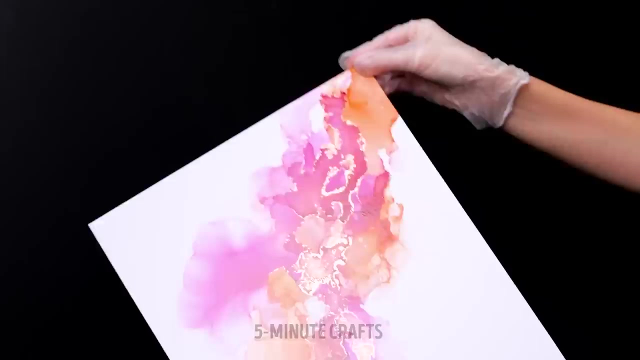 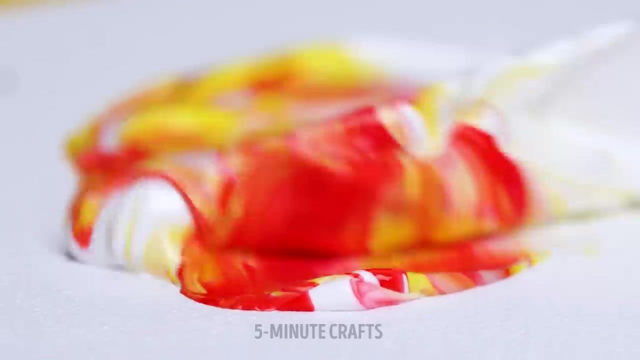 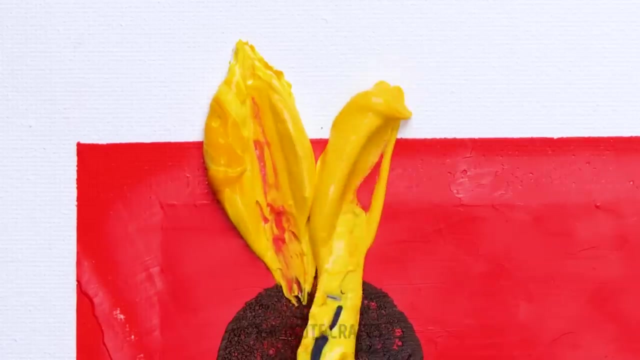 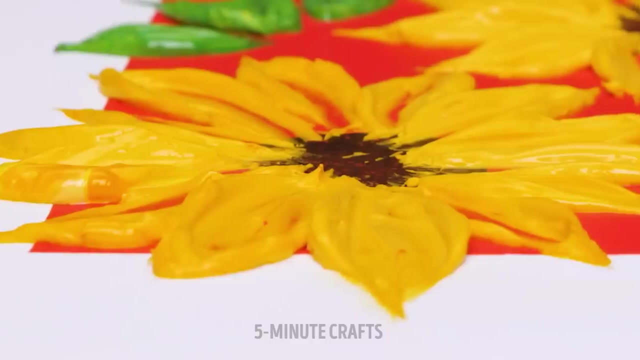 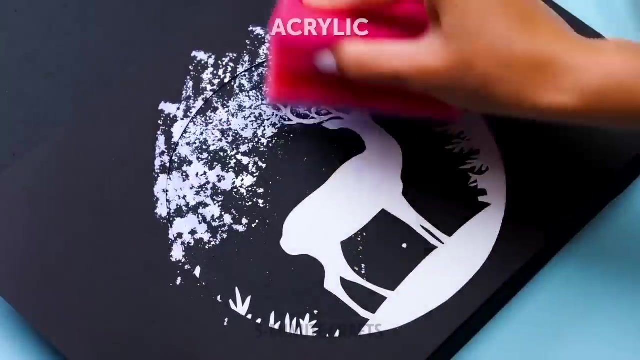 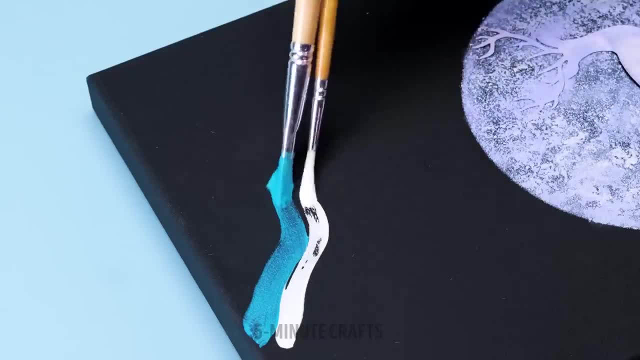 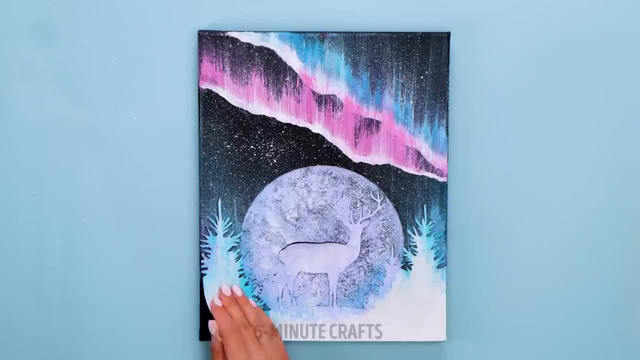 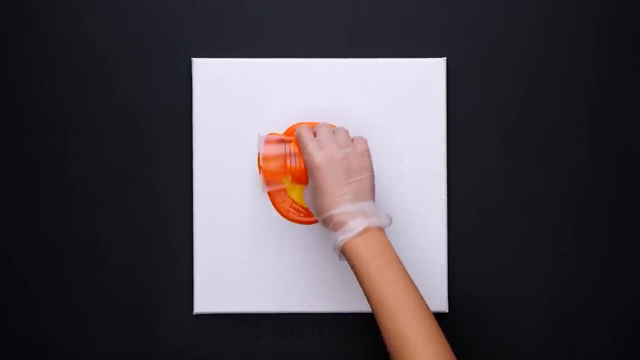 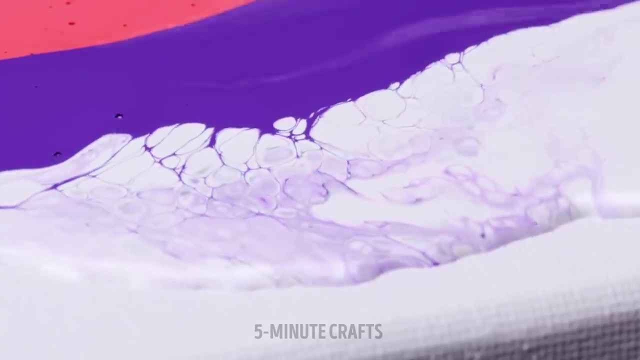 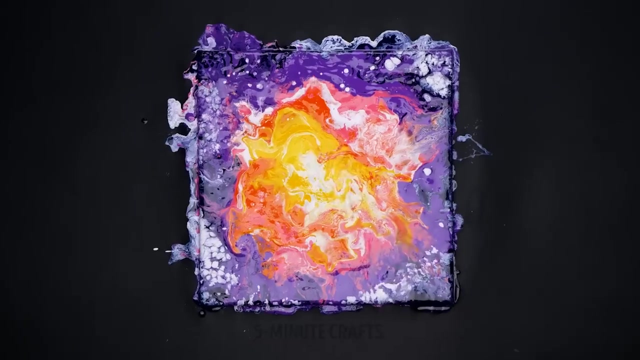 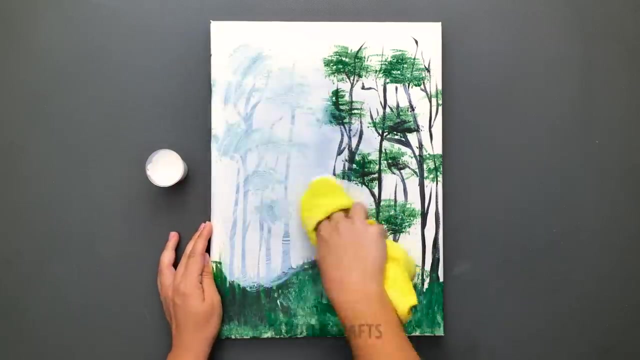 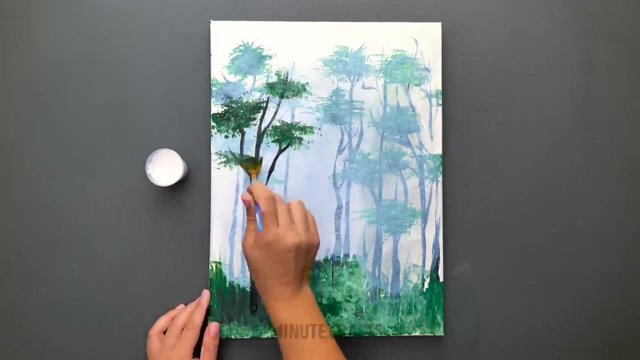 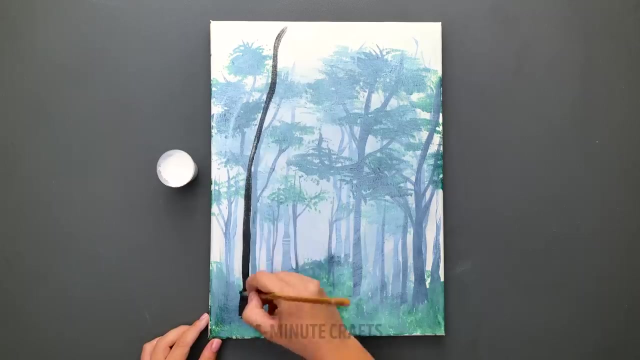 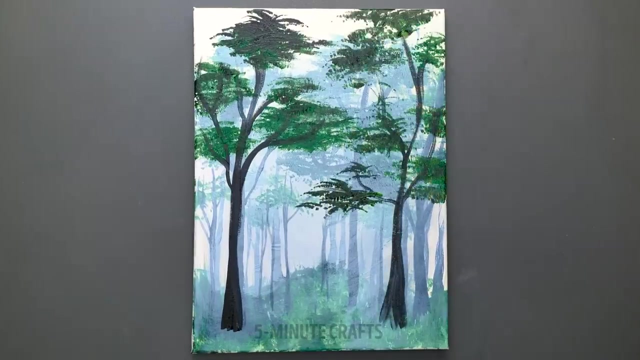 Thank you for watching. Thank you for watching, Looking for love in every corner. The hardest part is to not think it over. Is he the one? Could I find a better one? I think I could do better. Every relation is a struggle these days. Try to keep them alive, but we throw them away. 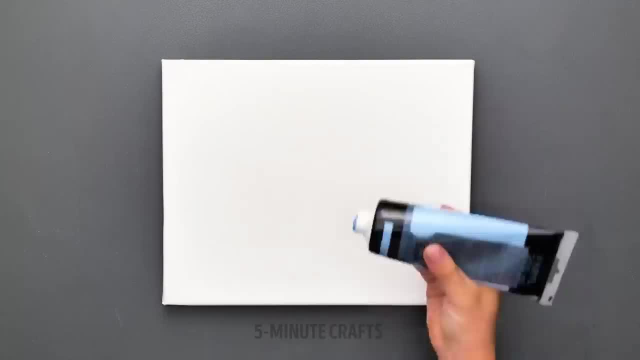 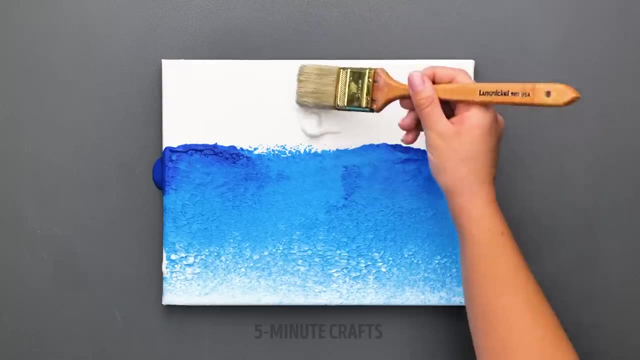 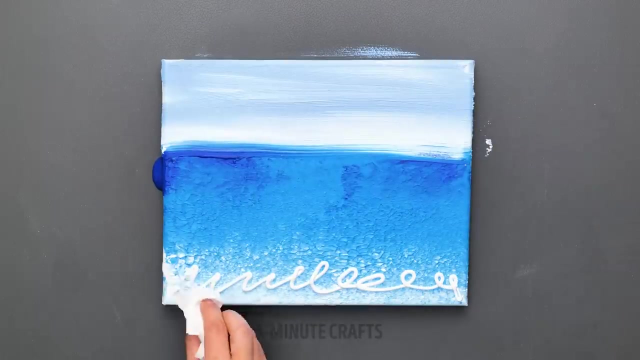 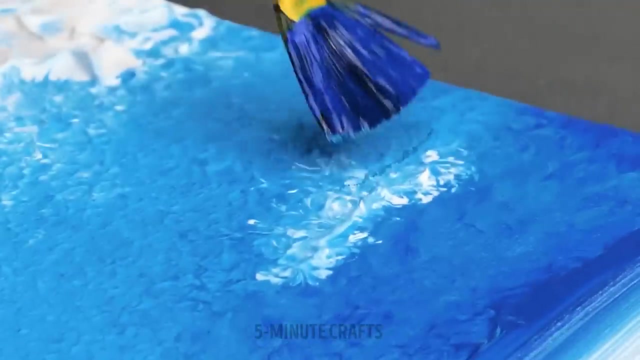 Oh, oh, oh. love should be a joy. Every relation is a struggle these days. Try to keep them alive, but we throw them away. Oh, oh, oh. love should be a joy. The moment you see me, you know what it feels like. 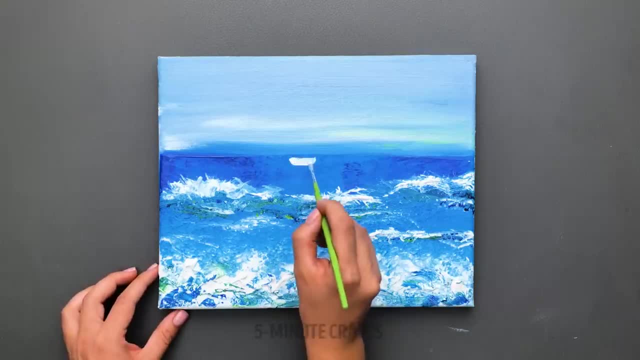 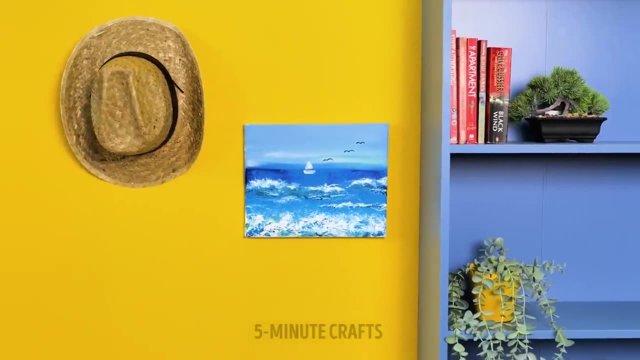 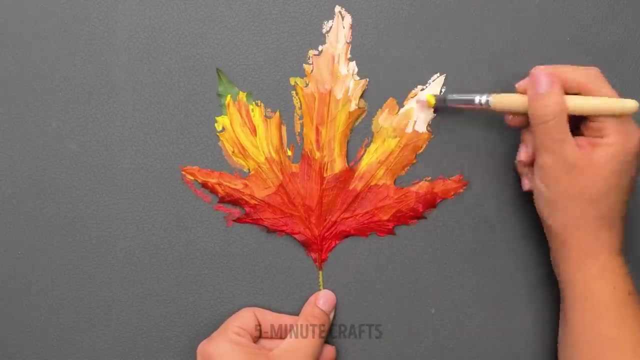 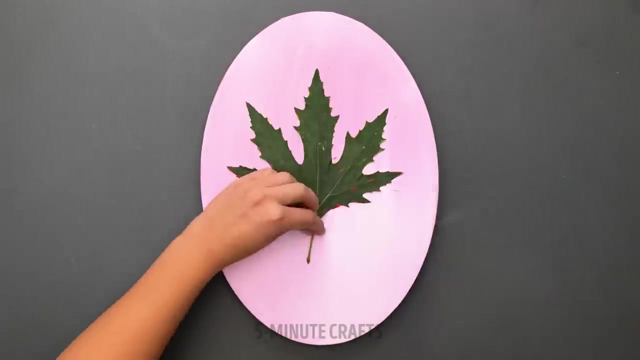 Yeah, but after a week something doesn't feel right. Is he the one? Could I find a better one? I think I could do better. Every relation is a struggle these days. Try to keep them alive, but we throw them away. Oh, oh oh. love should be a joy. 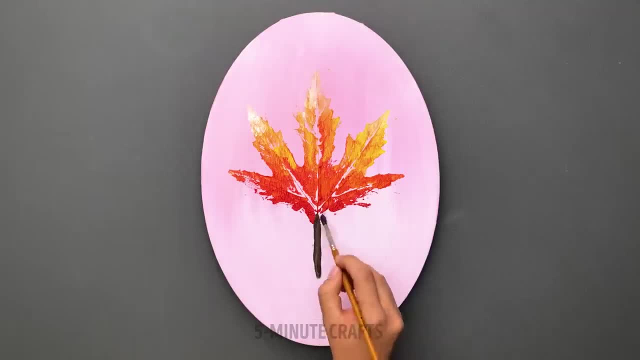 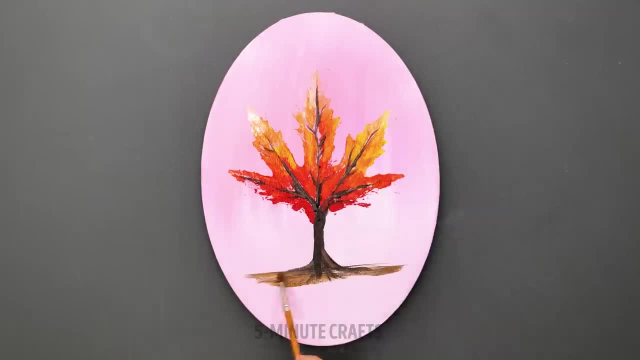 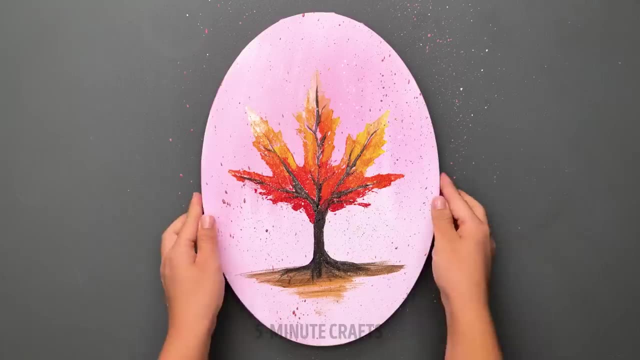 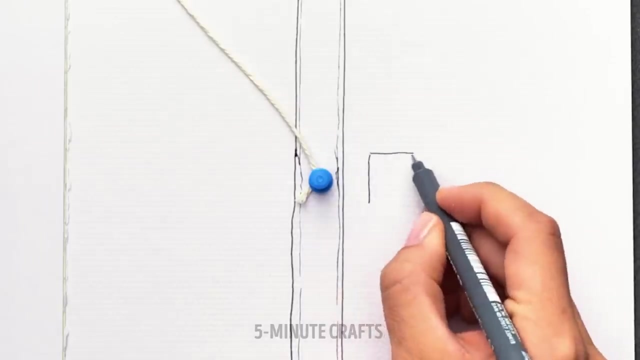 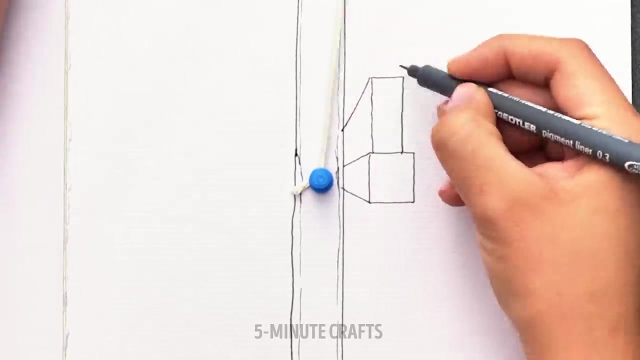 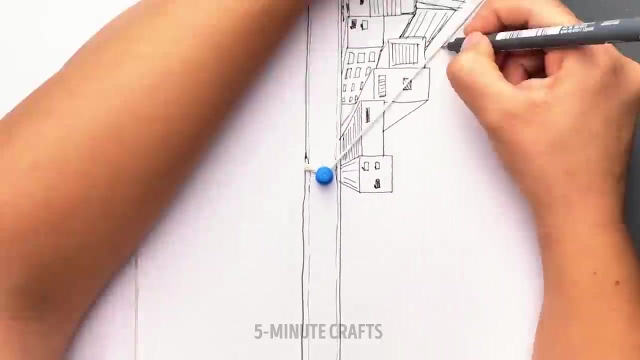 Every relation is a struggle these days. Try to keep them alive, but we throw them away. Oh, oh oh. love should be a joy. So many chances I have lost. It's not okay. It doesn't feel okay. So much heartache in his heart. 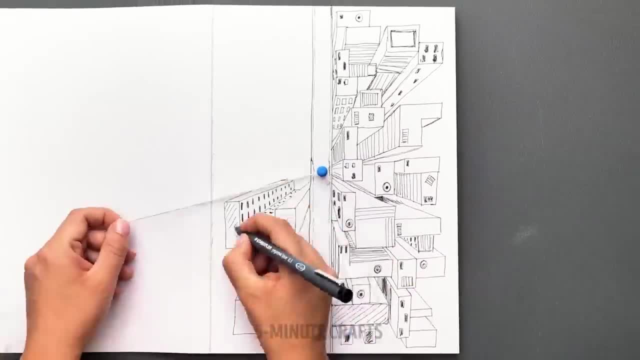 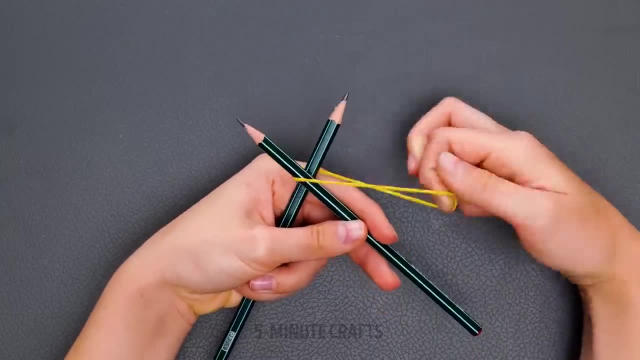 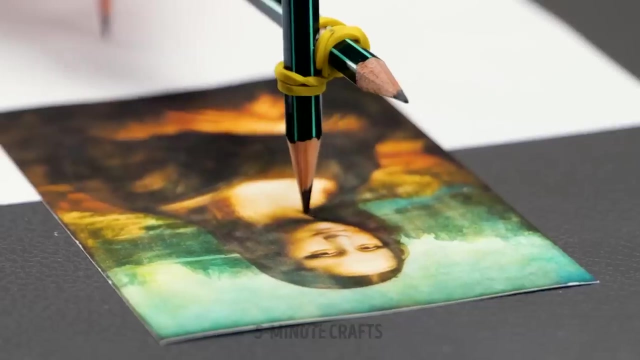 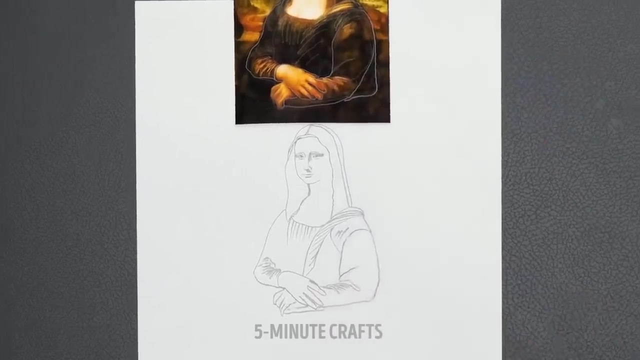 It's not okay, It doesn't feel okay. Every relation is a struggle these days. Try to keep them alive, but we throw them away. Oh oh oh. love should be a joy. Oh oh oh, love should be a joy. Every relation is a struggle these days. 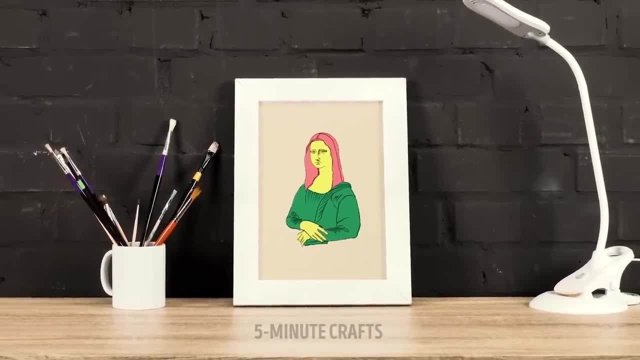 Try to keep them alive, but we throw them away. Oh oh oh, love should be a joy. Oh, oh, oh, love should be a joy. Every relation is a struggle these days. Try to keep them alive, but we throw them away. 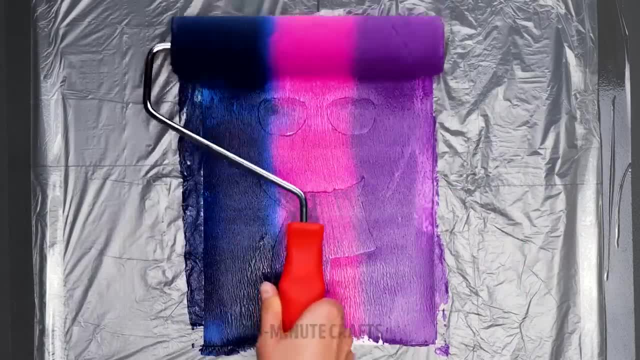 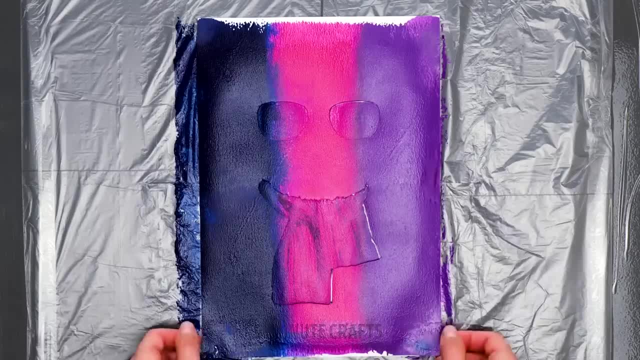 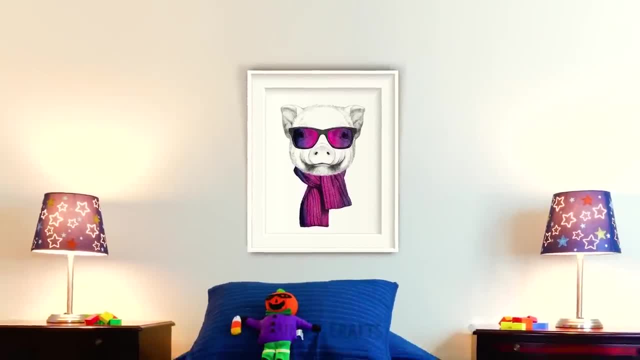 Every relation is a struggle these days. Try to keep them alive, but we throw them away. Oh, oh, oh, love should be a joy. Oh, oh, oh, love should be a joy. Oh, oh, oh, love should be a joy. 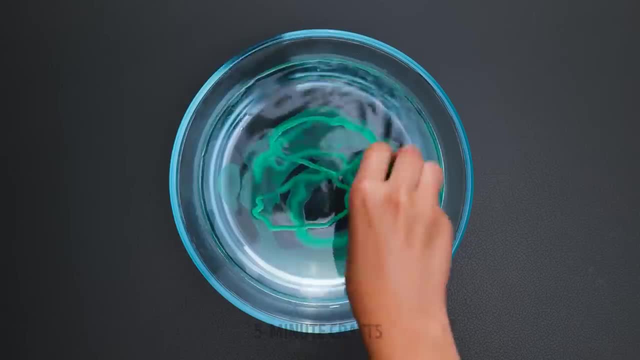 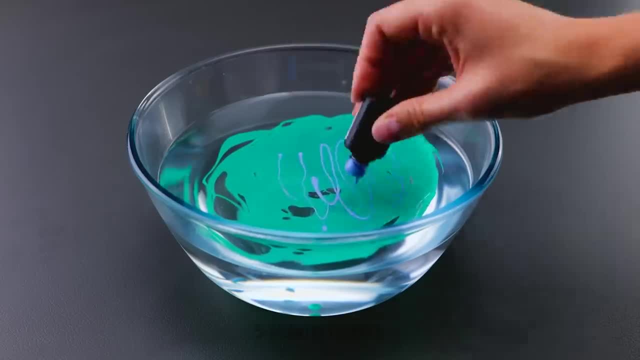 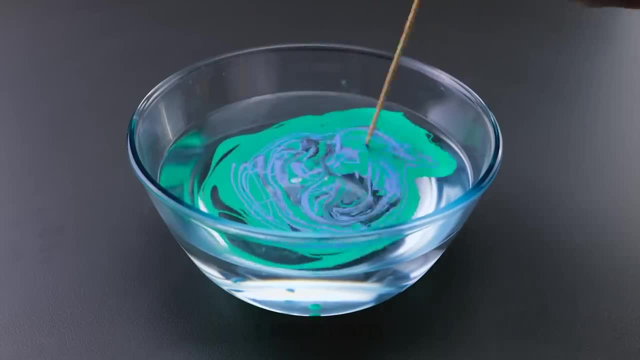 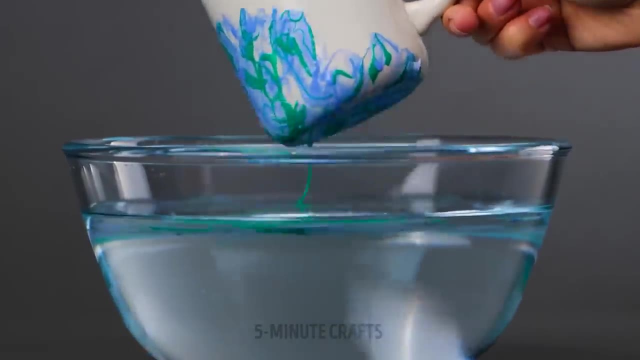 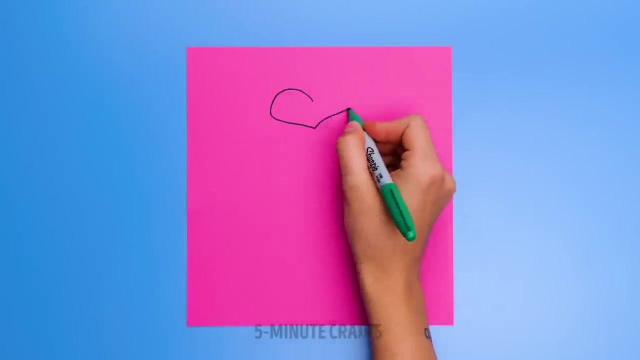 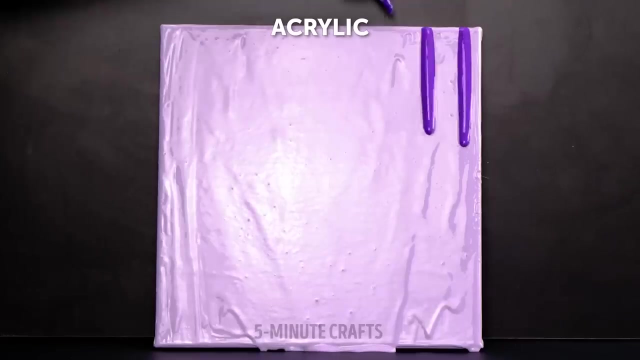 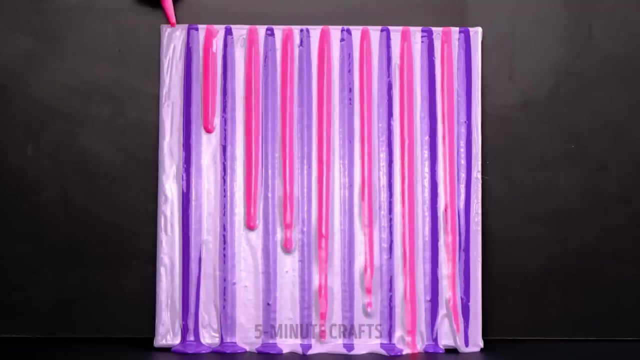 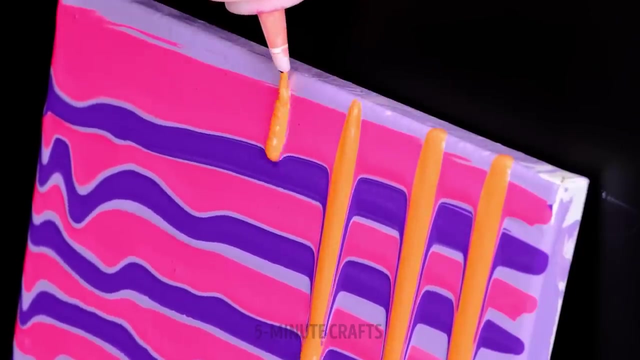 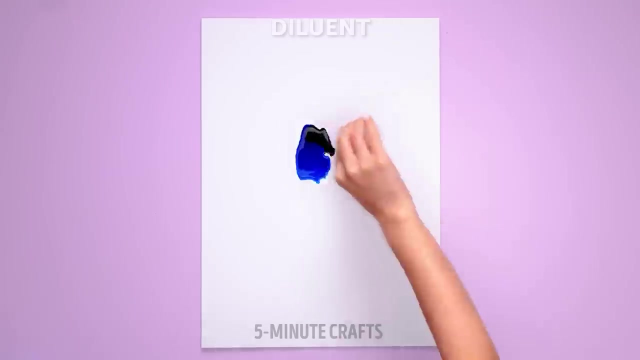 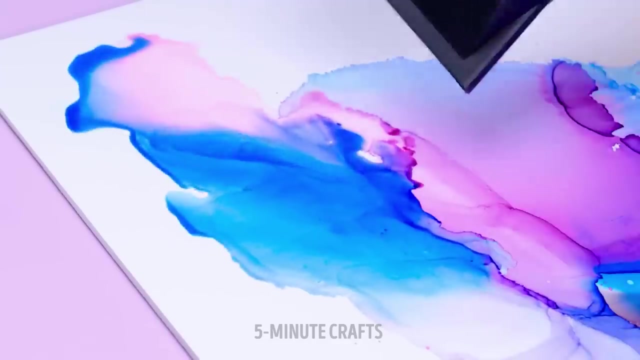 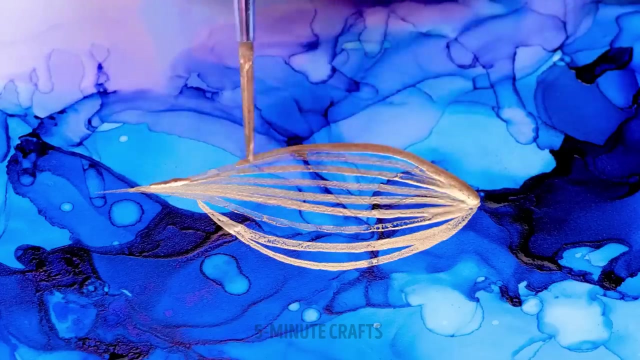 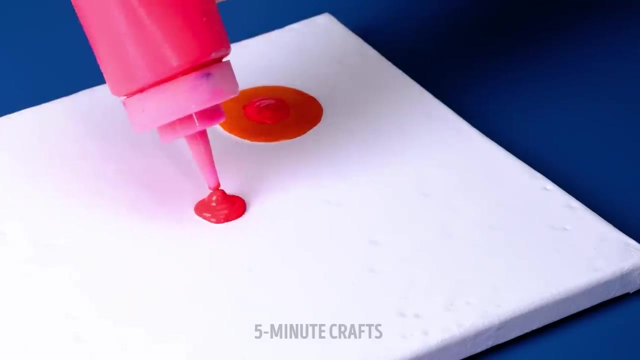 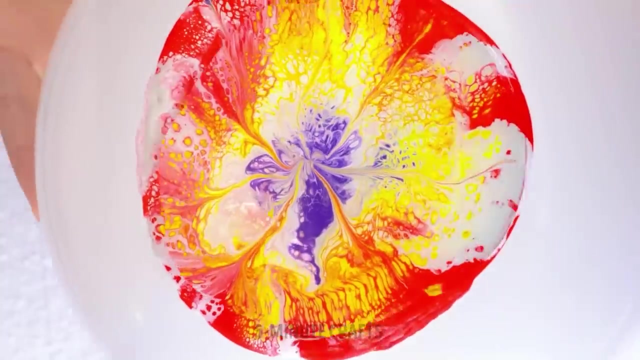 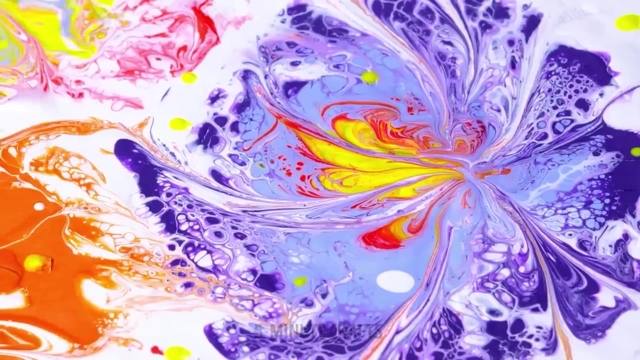 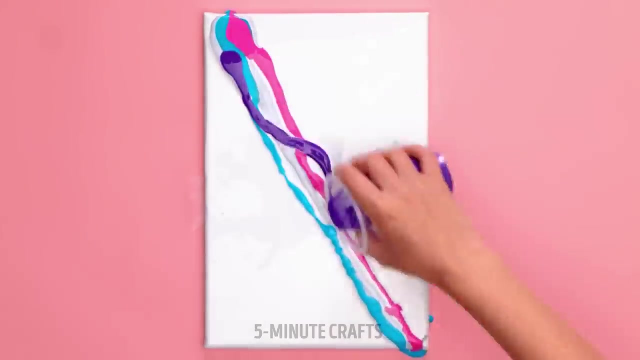 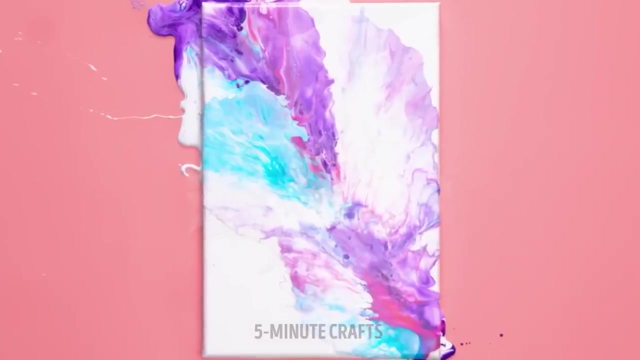 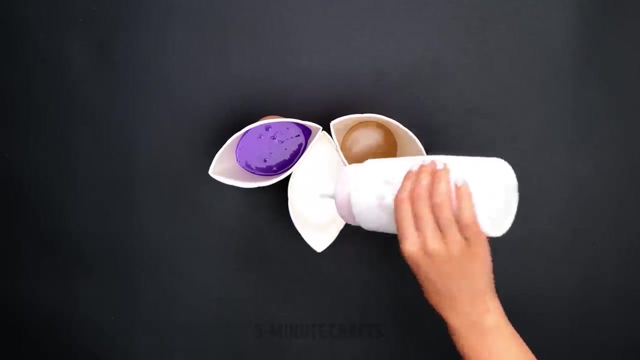 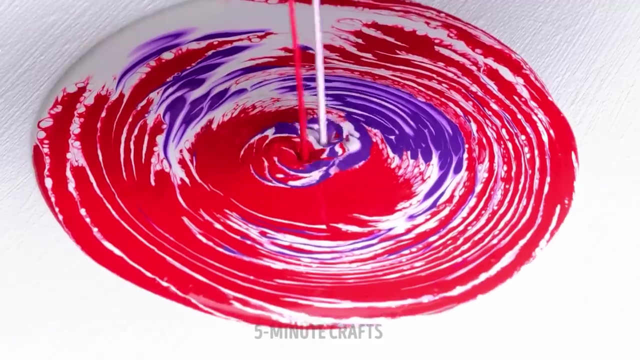 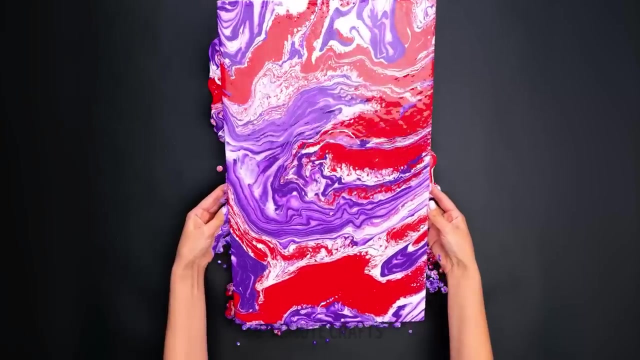 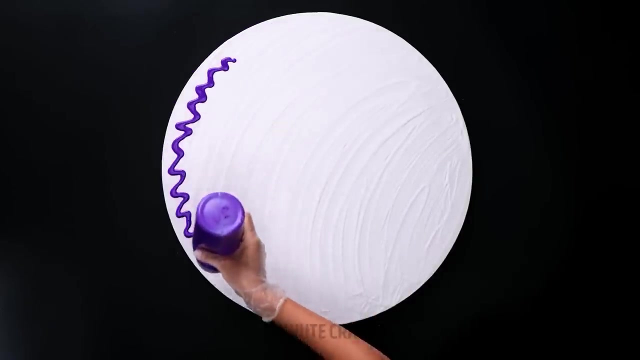 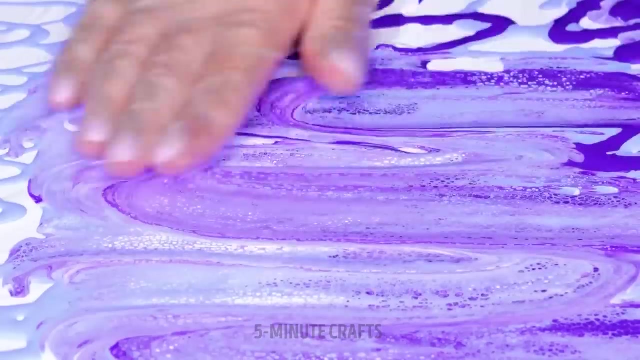 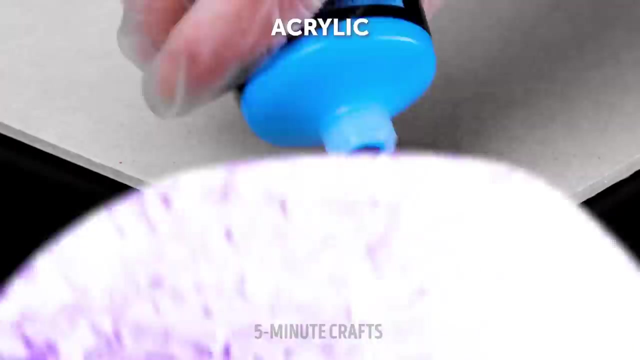 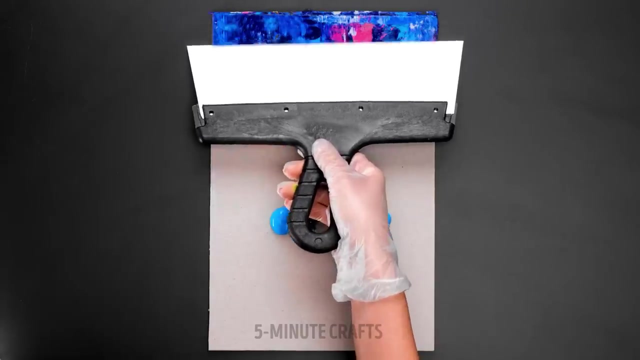 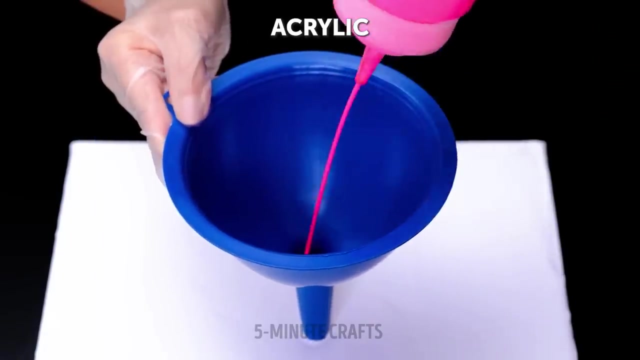 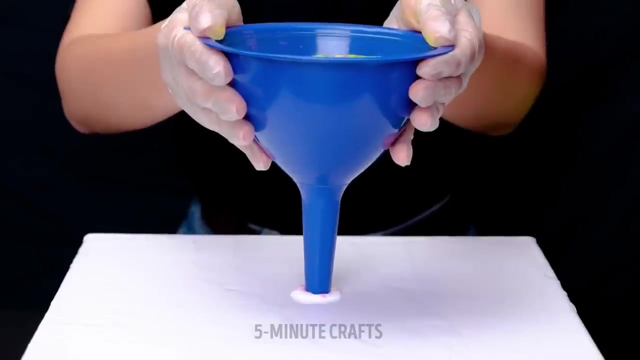 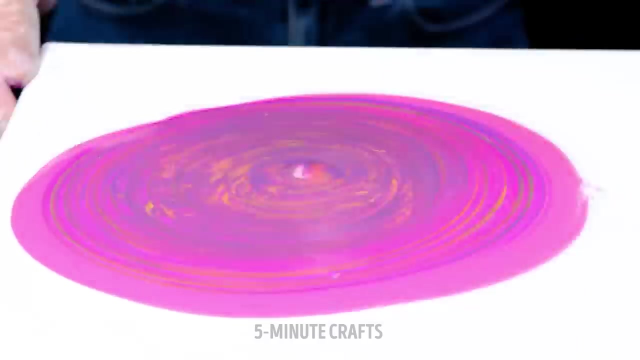 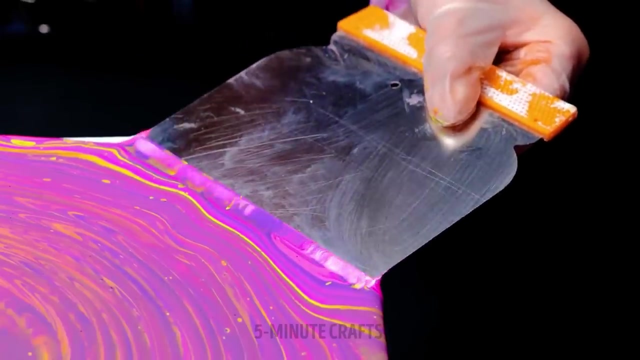